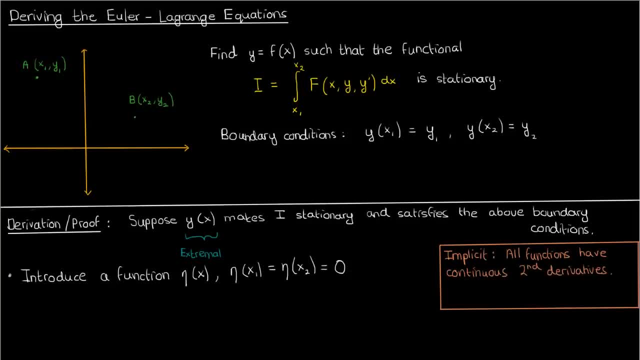 the functions we're concerned with all have continuous second derivatives, So just keep that in mind. Anyway, what we're going to do is define a new function, y-bar, given by our extremal y plus some parameter, epsilon times the arbitrary function eta. Essentially, y-bar represents a variation in the extremal y. 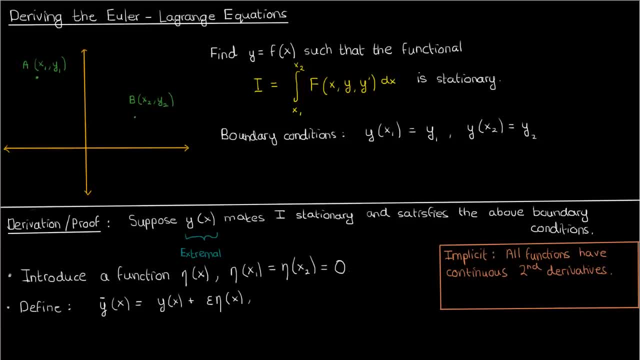 and because eta is an arbitrary function, you can conclude that, by extension, y-bar can also represent x2.. Now what we're going to do is find the particular curve in this family that makes our function stationary, and that's why we're going to use the y-bar function. 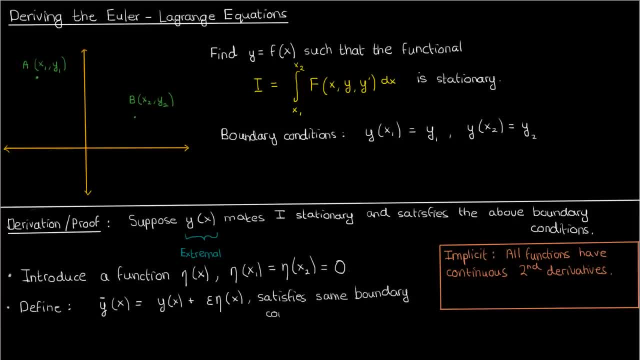 Now the y-bar function is a function that can be used to represent any arbitrary function. The only restriction on y-bar arises from the restrictions we put on y and eta earlier on, And you can easily verify that y-bar satisfies the exact same boundary conditions as y. Now, because of the parameter epsilon and 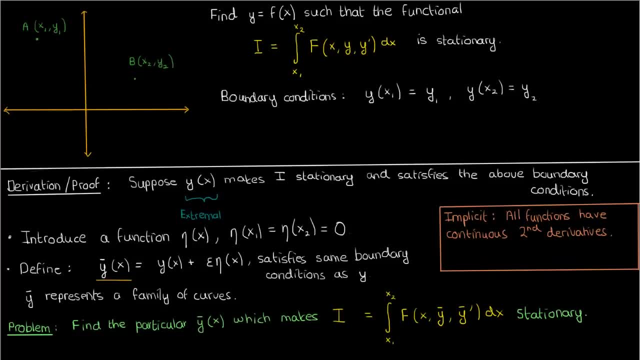 the arbitrary function eta. this y-bar can be interpreted as a non-discretionary function, So just remember that the only parameter that we can use is the quantity that makes our functional i stationary. Now, one thing I want you to notice before I continue is that this quantity i depends only on the parameter epsilon. 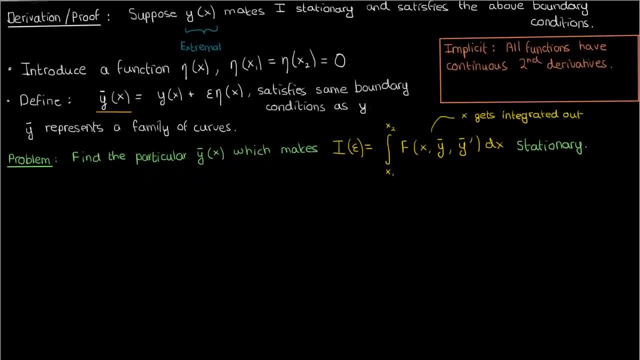 Why is that? Well, because the x gets integrated out from this definite integral, which means that once you integrate and apply your limits to end up with your i, the only parameter or variable remaining in the. Now, my primary objective here is to make i stationary, but since i only depends on 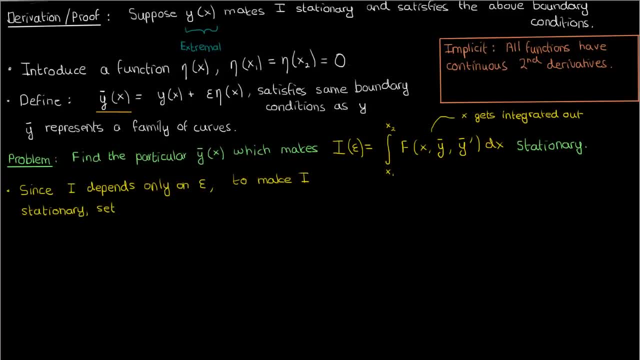 epsilon. making i stationary is equivalent to setting di d epsilon equal to zero. It's like single variable calculus. if you want a function to be stationary, just set its derivative to zero. But we already know what value of epsilon corresponds to a stationary i, and that's. 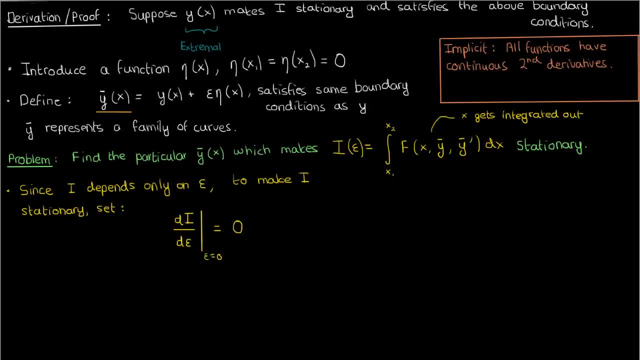 epsilon equals zero because, remember, the function y of x was already assumed to be stationary beforehand, and so it's easy to see that when epsilon equals zero, the particular curve that we end up for, y bar, is our desired extremal y. Alright, so what we're going to do is use this fact that di d epsilon equals zero at 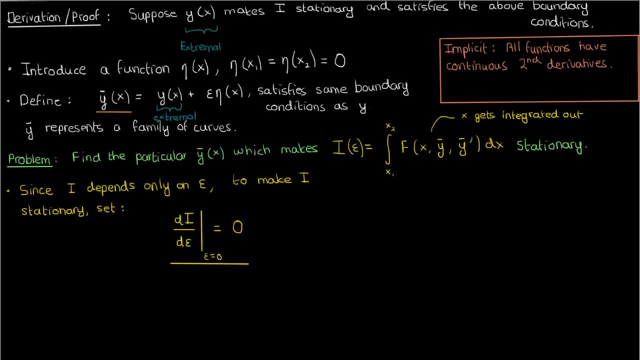 epsilon equals zero. we're going to use this fact to differentiate the integral expression, for i do some algebra and eventually arrive at the Euler-Lagrange equation. Hopefully, everything should be clear so far. Now, If the derivative of i with respect to epsilon is zero, then the derivative of this whole. 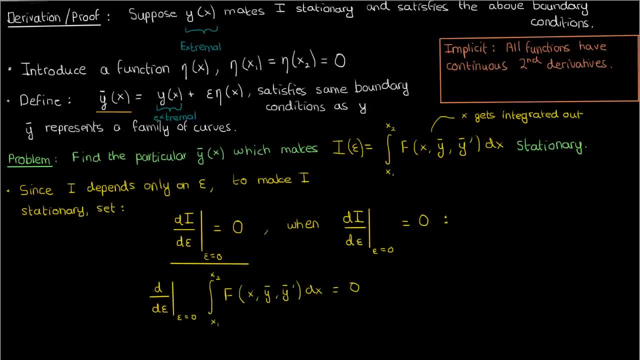 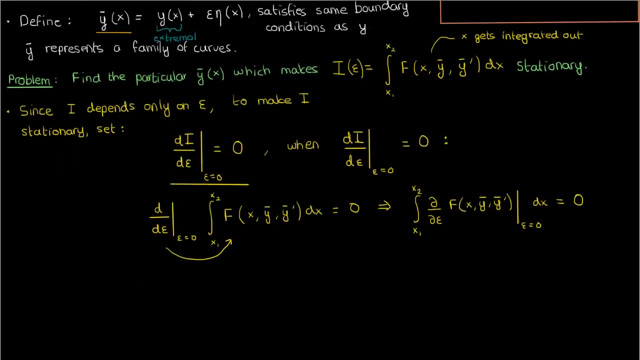 integral with respect to epsilon is zero, obviously because i equals this integral by definition. Now let's move this derivative inside, in which case we end up with a partial derivative with respect to epsilon. Now, y bar and y bar prime are the only variables or functions inside capital F which depend 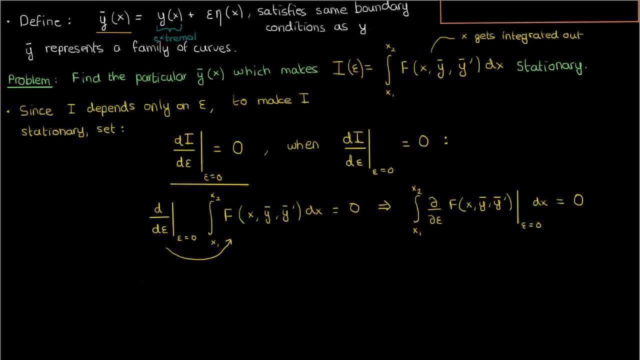 on. epsilon X is just an independent variable by itself, So what we can do is apply the chain rule of partial differentiation to end up with the integral from x1 to x2 of partial F, partial y bar times, partial y bar partial epsilon plus. 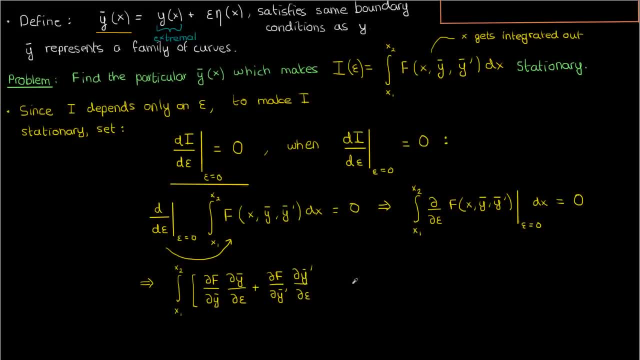 partial F, partial y bar prime times. partial y bar prime partial epsilon. And this integral at epsilon equals zero, has to be equal to zero. Let's copy paste the expression for y bar that we defined above, which is just: y bar equals y plus epsilon times eta. Now we also need to find the derivative of y. 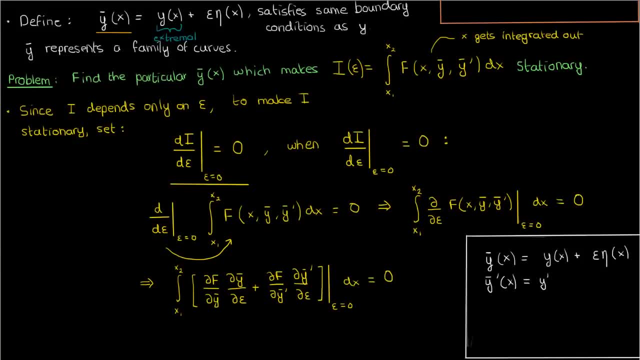 bar, y bar prime, and the derivative of y bar is then just given by y prime x plus epsilon times eta prime x. If I take the partial derivatives of these expressions with respect to epsilon now, then I'll end up with eta and eta prime. 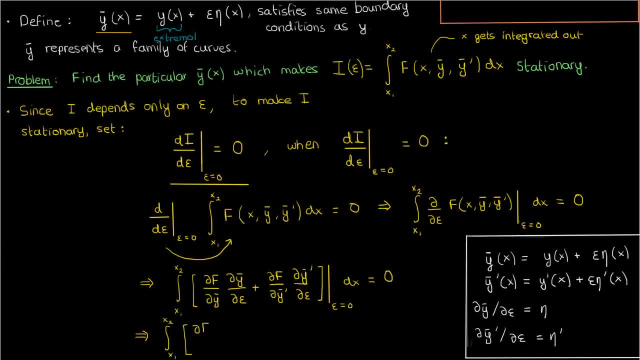 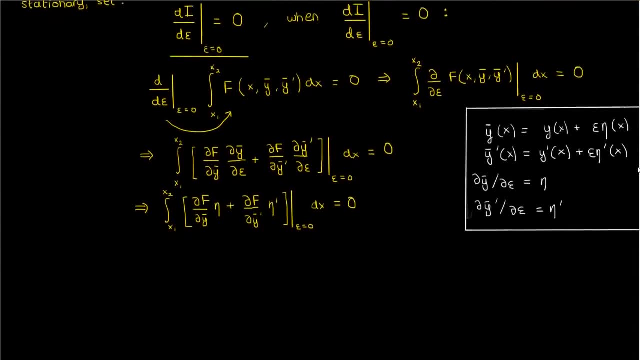 respectively, And let's plug them back into our expression for di d epsilon, and this is what we'll end up with. Alright, so now we need to simplify further. We'll take the second term in this integral and integrate it by parts separately. 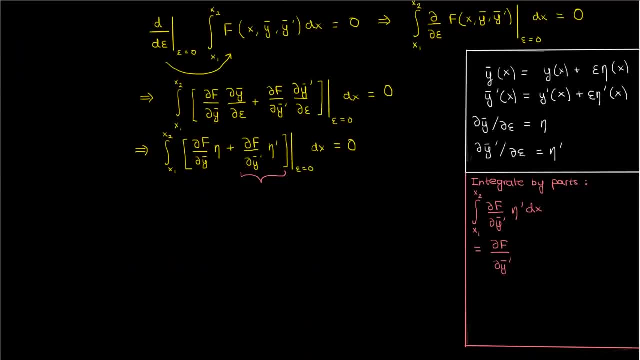 We'll have the first function, which is the partial of capital F with respect to y bar prime times the integral of eta prime with respect to x, minus the integral of the integral of eta prime times the derivative, with respect to x, of partial F, partial y bar prime, And, of course, our limits of x1 and x2 would 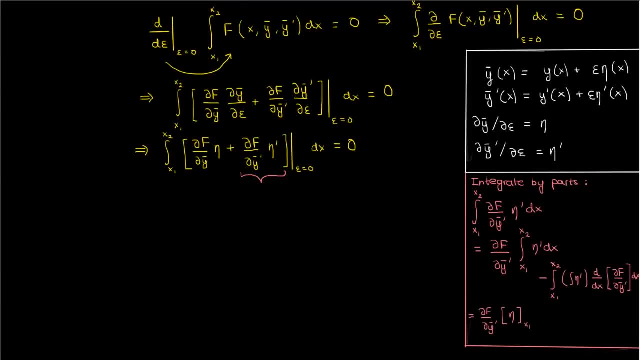 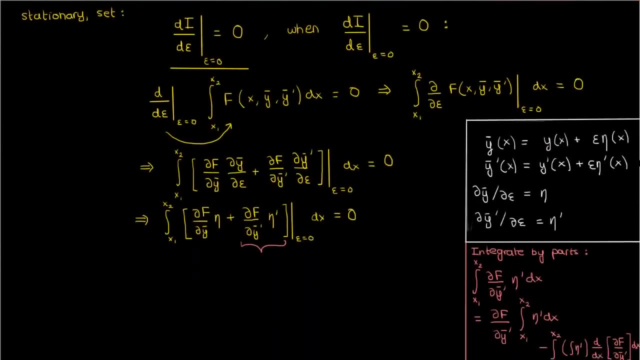 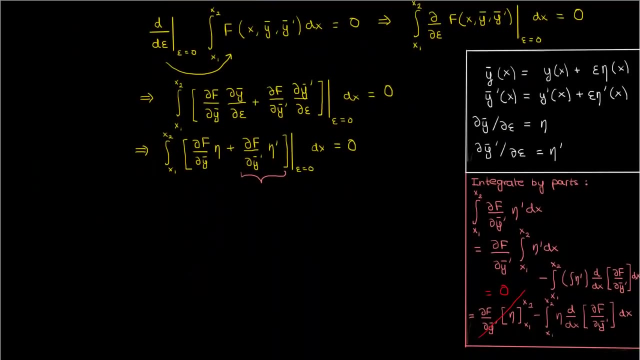 still be the same. The integral of eta prime is just eta, so let's just plug that in. Now we know from the boundary conditions on eta that at both x1 and x2, eta is just 0, so we can cancel out this first term in the integration by parts expression. And